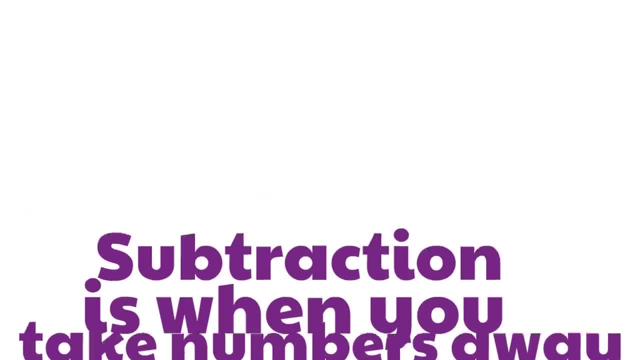 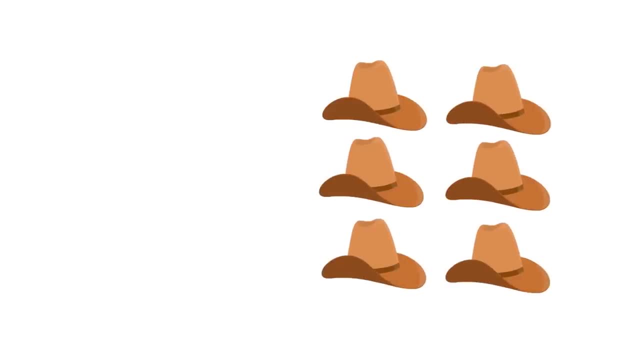 is when you take numbers away. Let's say, I have six hats and there's no way that I need six hats that look exactly the same. Well, good news: Two of my friends need hats and I decide to give two of my. 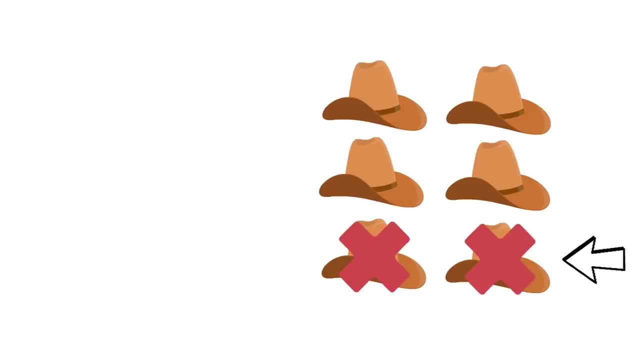 hats away. When you take numbers away, remember that is subtraction. If we were to write it out, it would look like this: Six minus two. So how many hats do I have now if I take two away? Yes, the answer is four. I have four hats now. 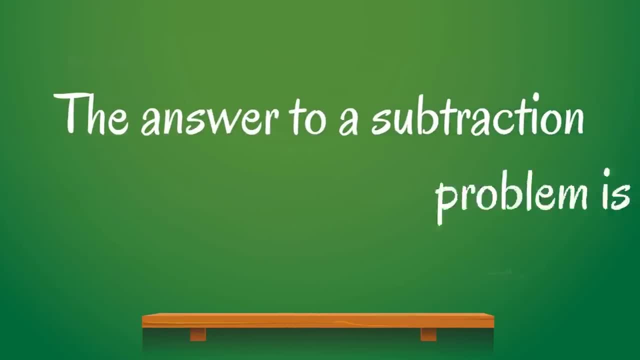 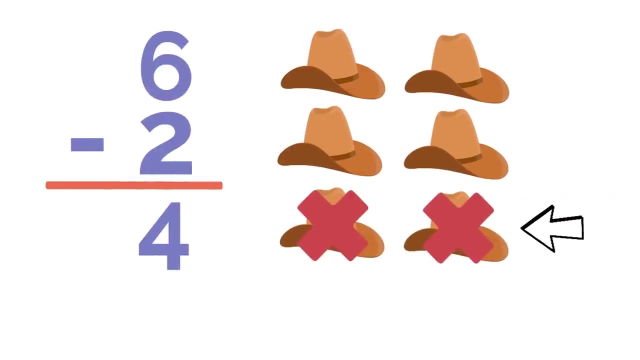 Now this is interesting. The answer to a subtraction problem is called the difference. Can you say that with us, The difference? Yeah, the answer to a subtraction problem is called the difference. That means, in our example, the difference is four. 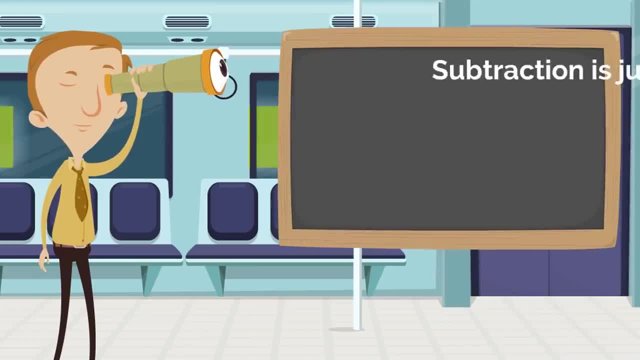 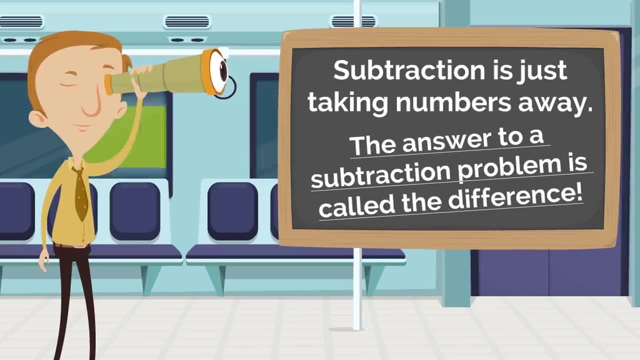 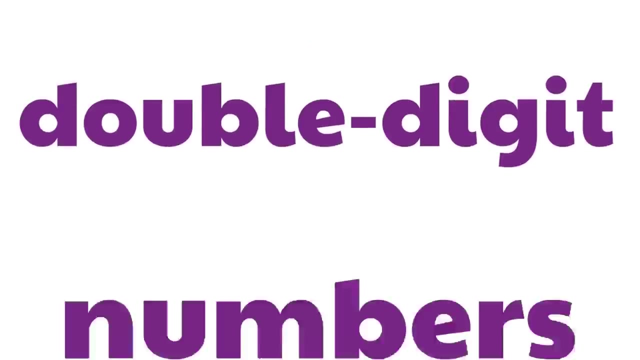 So subtraction is just taking numbers away and the answer to a subtraction problem is called the difference. Now that we have that, we want to look at bigger numbers, Double digit numbers. Let's say we have a lot of blueberries. For some reason they're just. 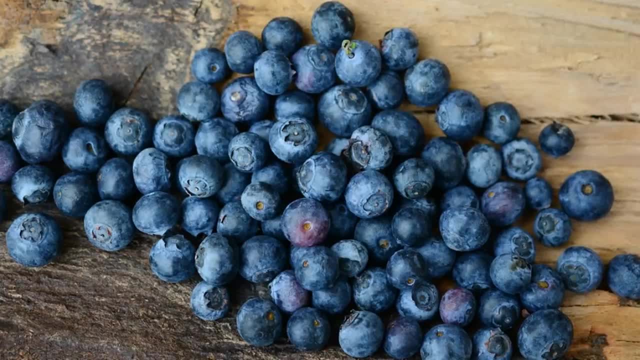 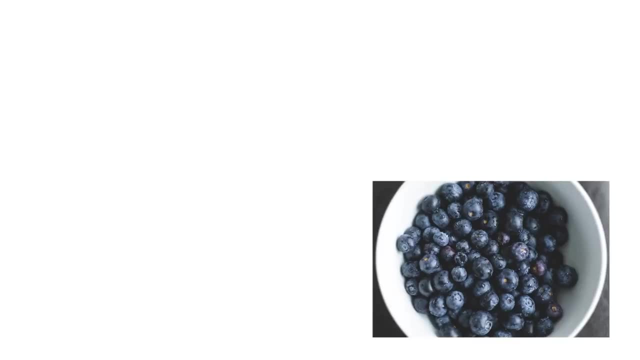 hanging out on a wooden table. We need to wash them and put them in a bowl. Let's pretend that when we were putting them in the bowl, we counted them and found that we had 66 blueberries. That's a lot of blueberries. You and your friends are hungry and blueberries are. 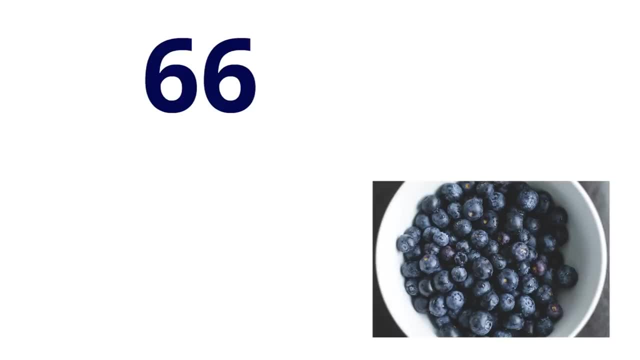 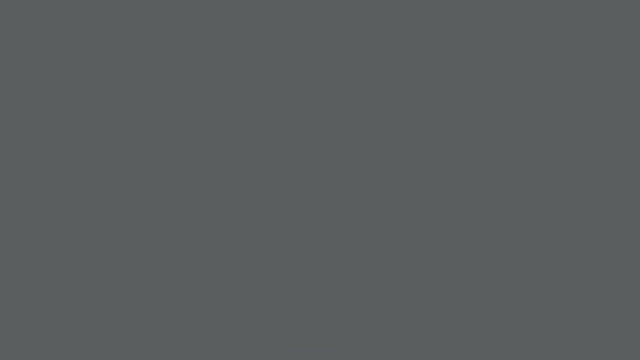 super yummy, right? You and your friends eat 54 blueberries. That's right. These are some big numbers, some double-digit numbers. To find out how many blueberries we have left, we simply subtract 54 from 66.. Let's look at how that's done. Here is our subtraction problem again. 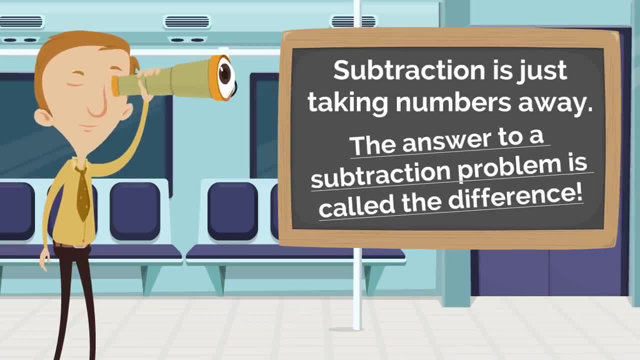 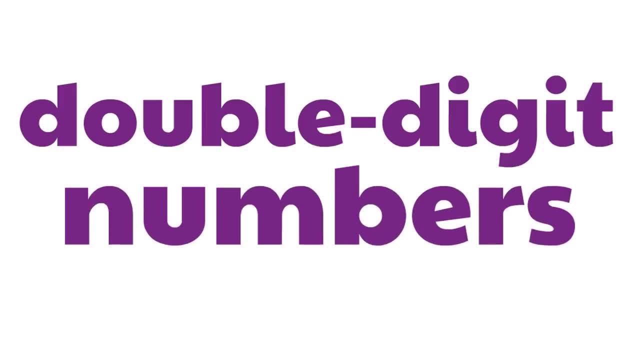 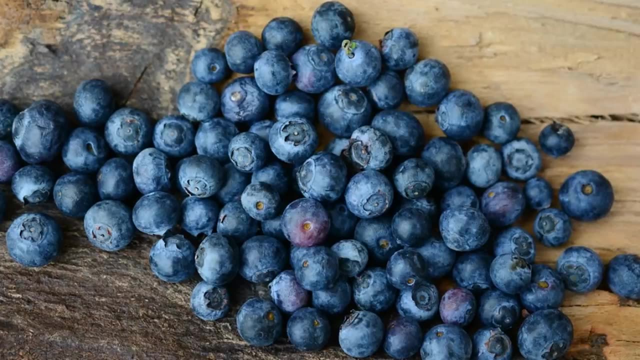 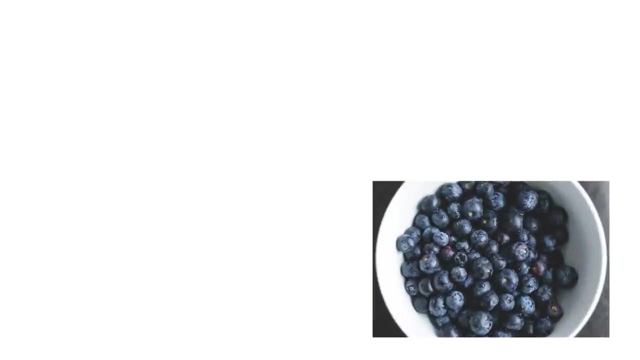 called the difference. Now that we have that, we want to look at bigger numbers, Double digit subtraction numbers. Let's say we have a lot of blueberries. For some reason they're just hanging out on a wooden table. We need to wash them and put them in a bowl. Let's pretend that when we were putting 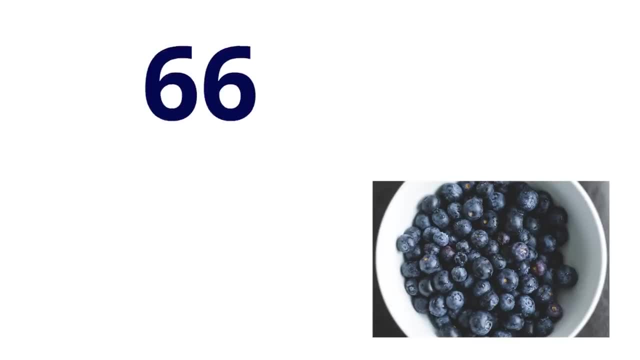 them in the bowl. we counted them and found that we had 66 blueberries. That's a lot of blueberries. You and your friends are hungry and blueberries are super yummy, right? So you and your friends eat 54 blueberries, That's right. These are some big numbers, some double digit numbers, to find out. 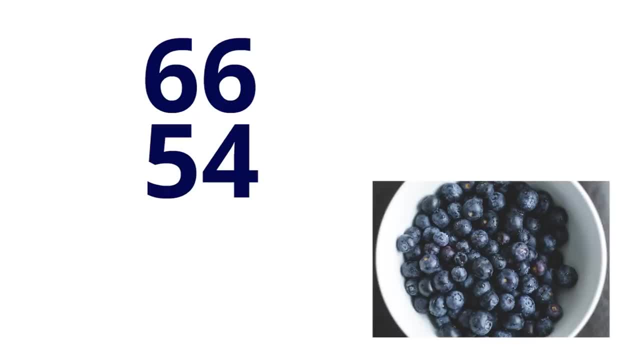 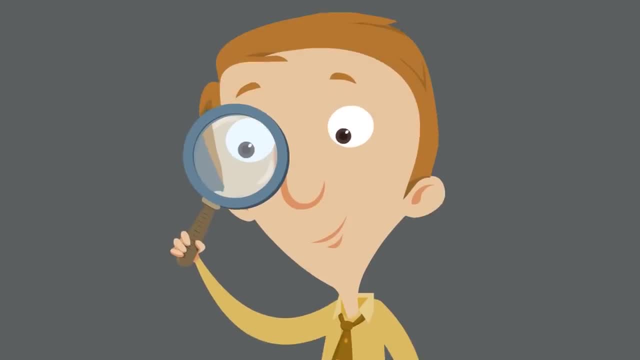 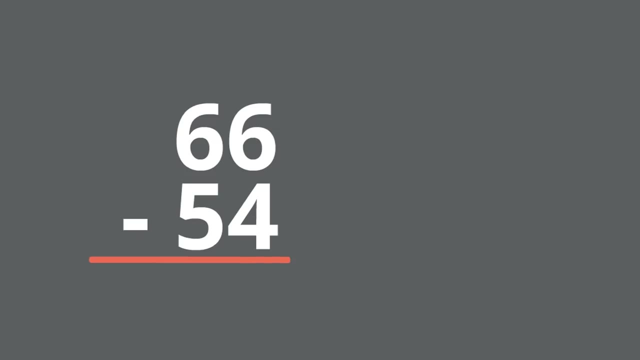 how many blueberries we have left. We simply subtract 54 from 66.. Let's look at how that's done. Here is our subtraction problem again: 66 minus 54 with double digit subtraction. All we do is break this down. We have a lot of blueberries. We have a lot of blueberries. We have a lot of blueberries. 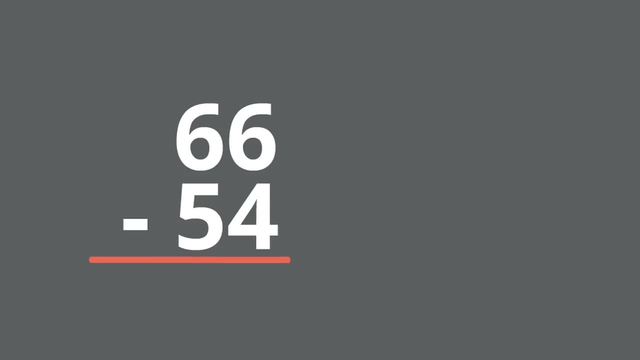 Big problem up into two little problems. First, we will subtract the right column, the ones To make it a little easier. we are going to cover the tens column with this blue rectangle. Suddenly, this big subtraction problem is a really easy one. What is six minus four? Do you know? Yes, six minus four. 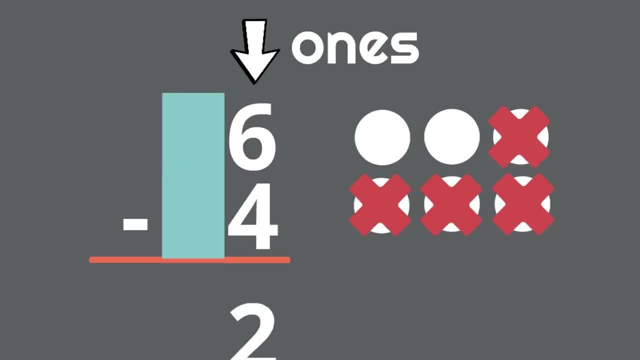 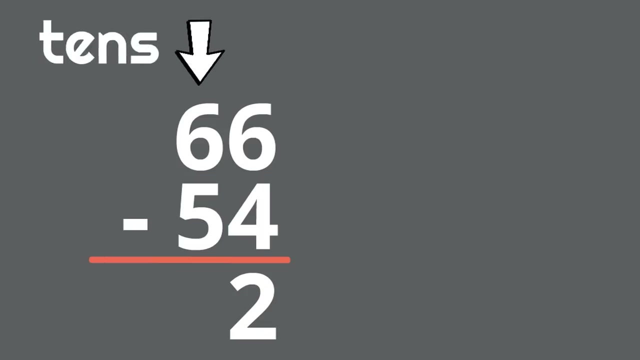 equals two. So we put the number two under the number two, We put the number two under the number two. We put the number two under the one's column, the right side. Great job, We are halfway to our answer. Next we will subtract the left column, the tens, And this time we're going to cover up the ones. 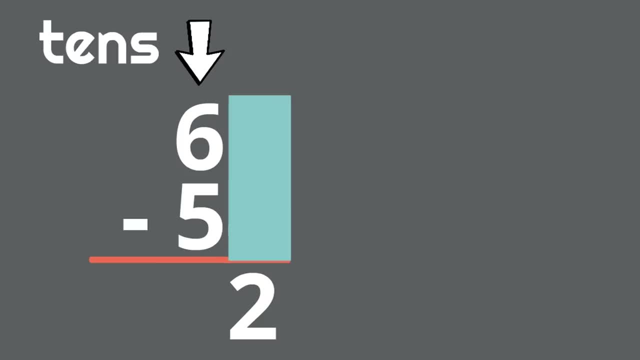 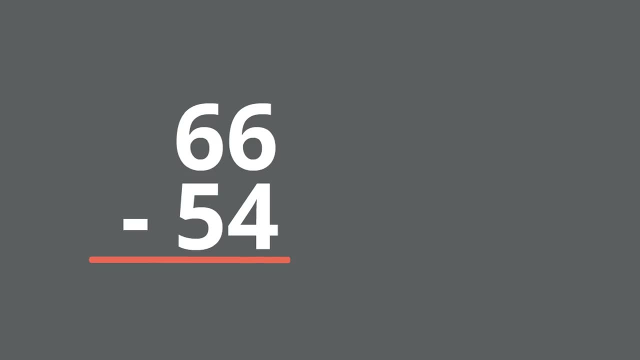 66 minus 54. With double-digit subtraction, all we do is break this big problem up into two little problems. First we will subtract the right column, the ones To make it a little easier. we are going to cover the tens column with this blue rectangle. Suddenly, this big subtraction problem is a really 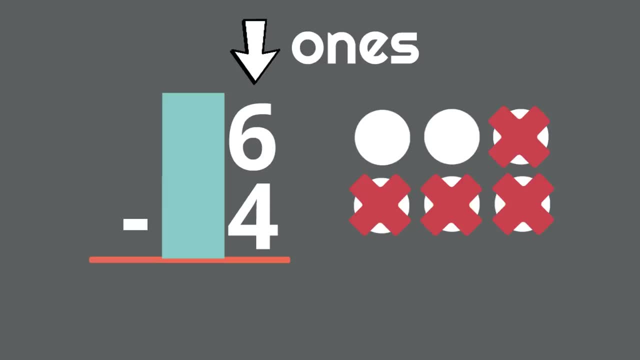 easy one. What is 6 minus 4?? Do you know? Yes, 6 minus 4.. 6 minus 4 equals 2.. So we put the number 2 under the ones column, the right side. Great job, We are. 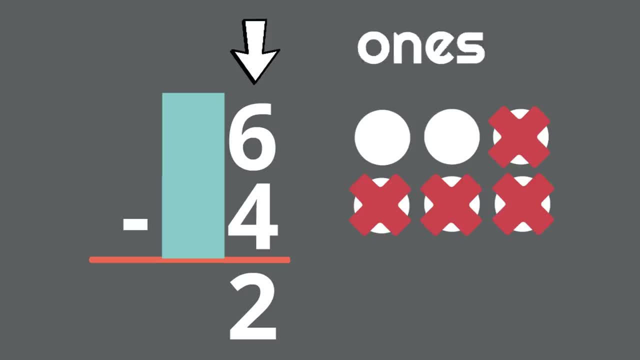 halfway to our answer. Next, we will subtract the left column, the tens, And this time we're going to cover up the ones column to make it a little easier. So what is 6 minus 5? 6 minus 5.. 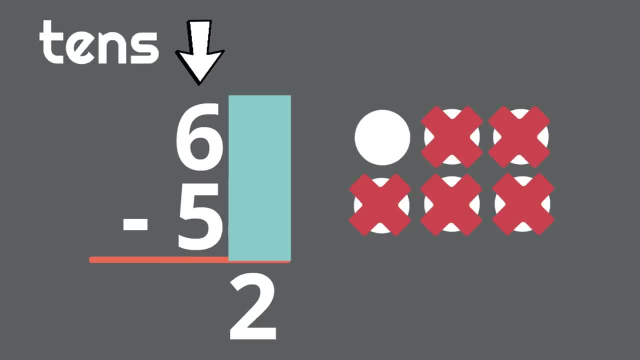 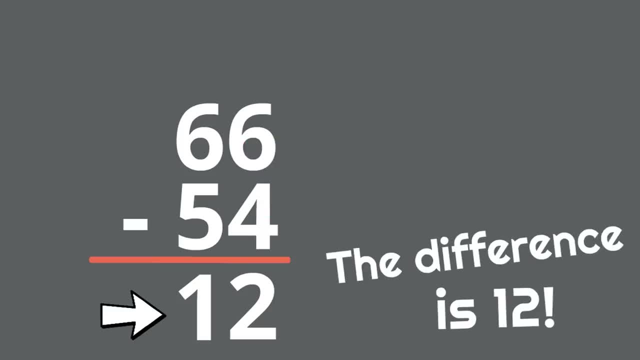 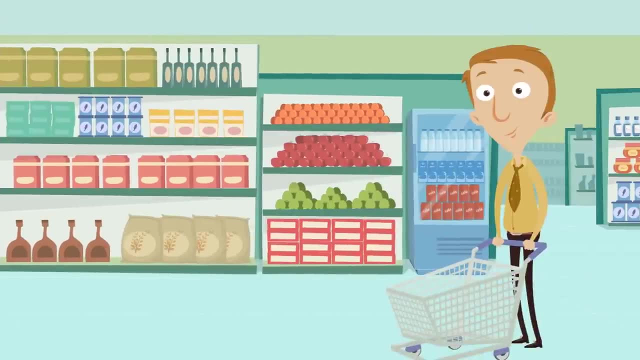 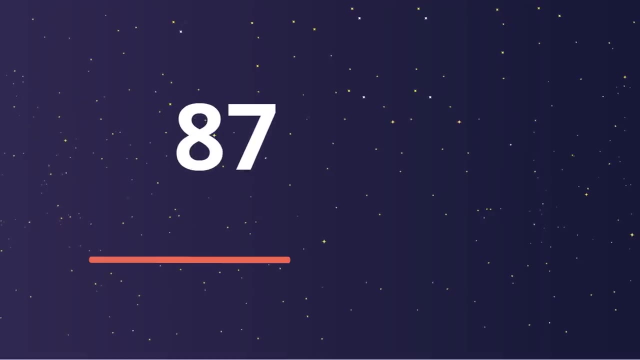 our answer: The difference is 12.. There are now just 12 blueberries. All right, let's do another one. How about 87 minus 53?? This should be fun. First subtract the right side, the ones. What is 7 minus 3?? 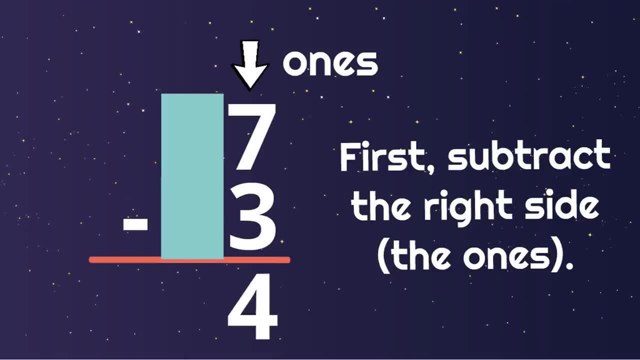 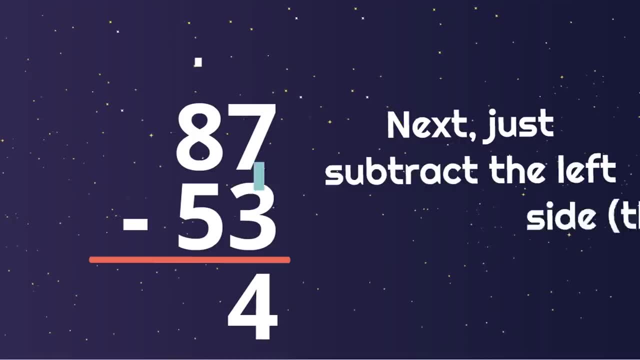 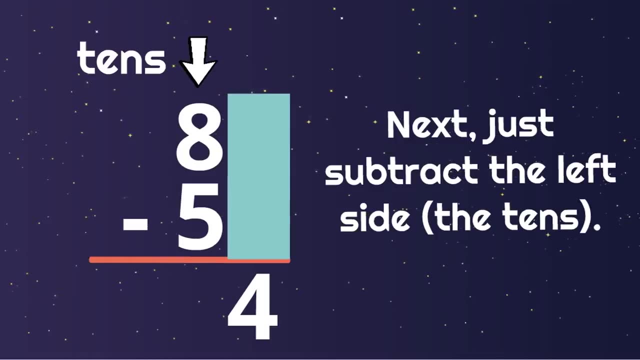 Yes, 4.. So we will write 4 under the ones. Simple. Next we just subtract the left side, the tens. What is 8 minus 5?? Yes, 3.. So we write 3 under the tens column. 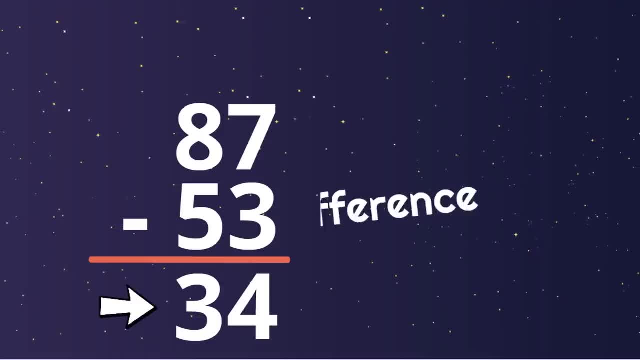 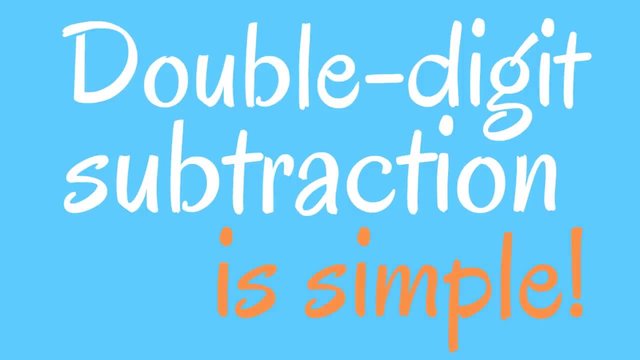 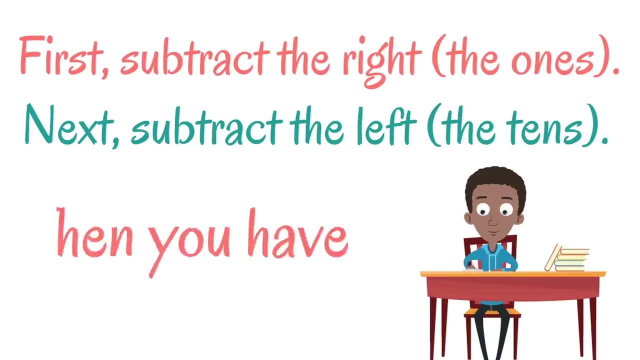 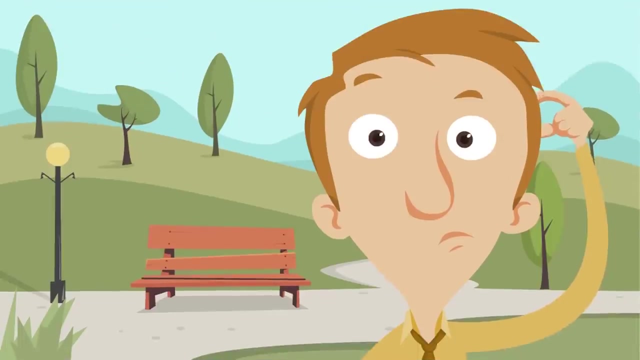 And we have our answer. The difference is 34.. Double digit subtraction is simple: First subtract the right, the ones, Next subtract the left, the tens. Then you have your answer, which is also called the difference. Now there is something interesting that can happen when you subtract larger numbers. 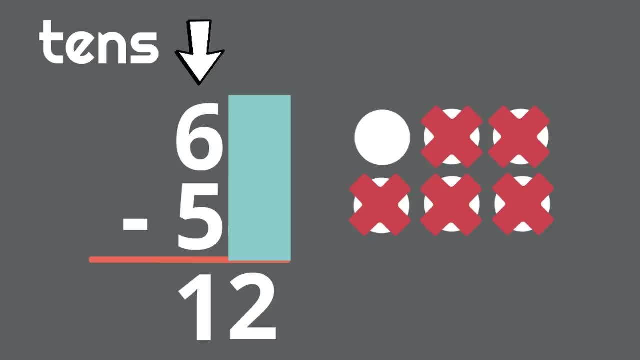 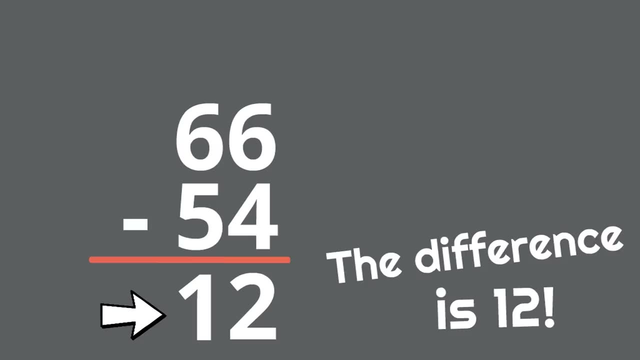 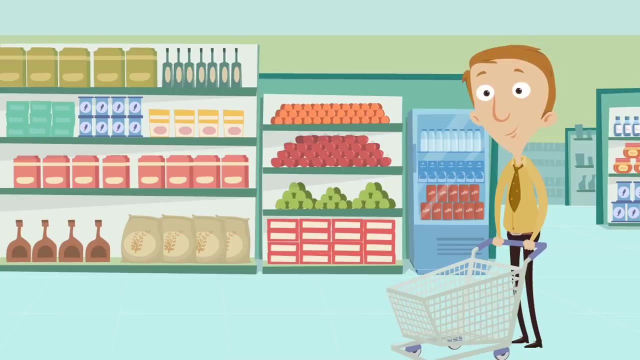 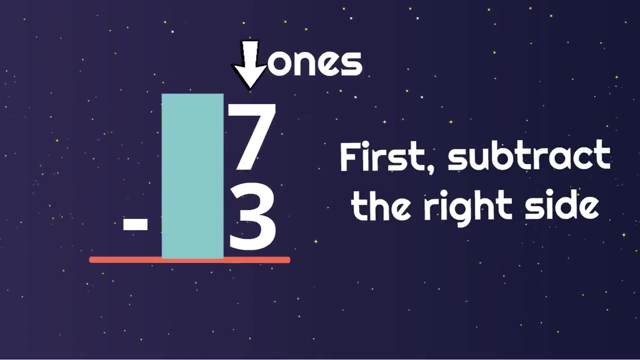 one under the tens, the left column, And just like that we have our answer. The difference is 12.. There are now just 12 blueberries. All right, let's do another one. How about 87 minus 53?? This should be fun. First, subtract the right side, the ones. What is seven? 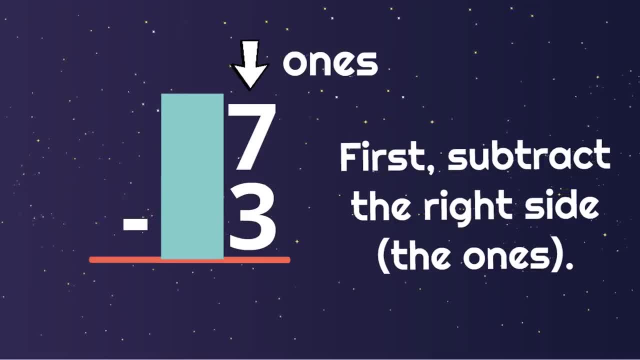 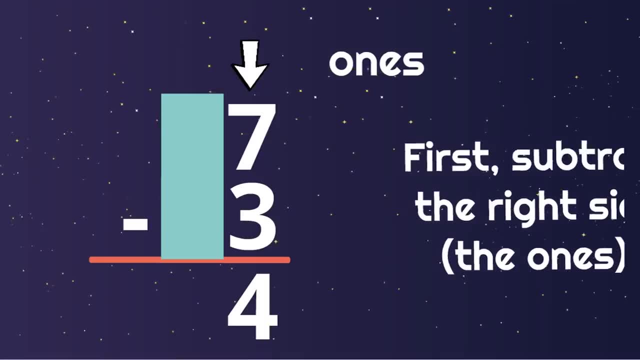 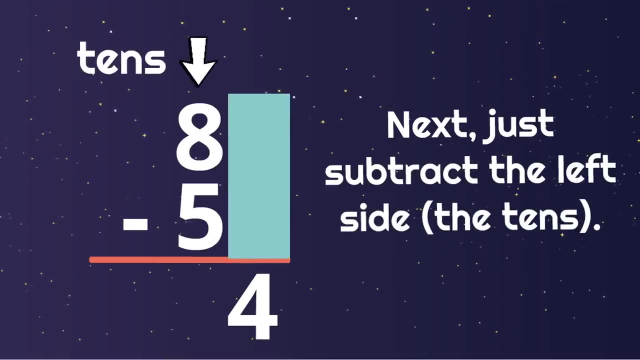 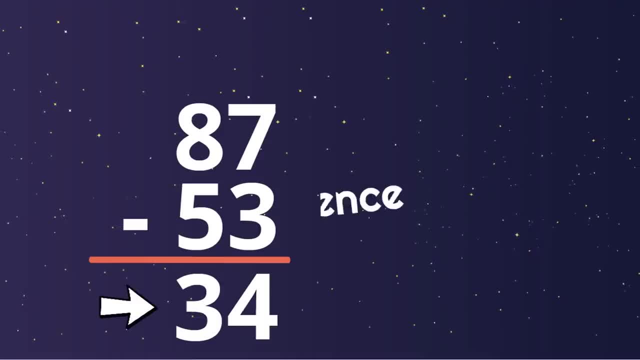 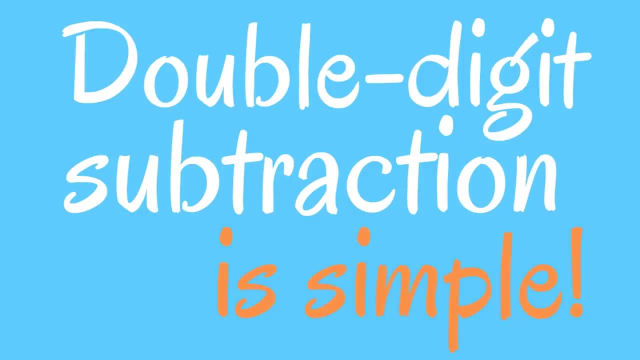 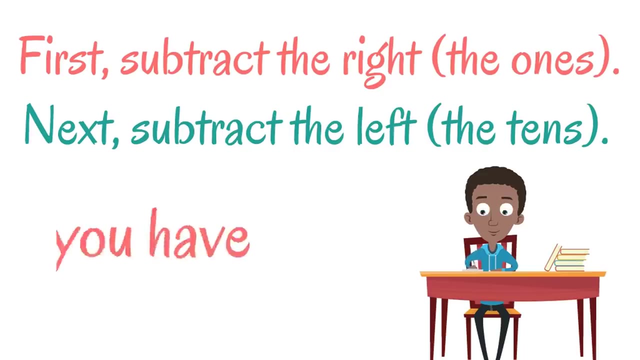 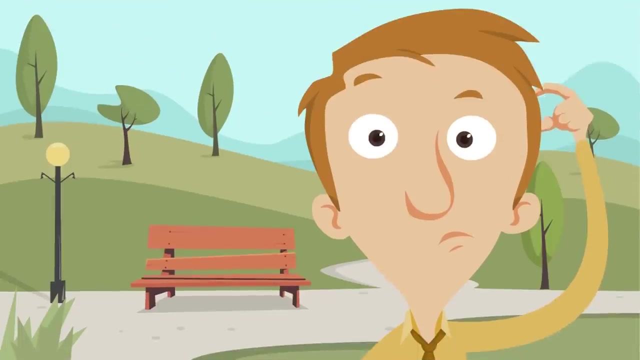 And we have our answer. The difference is 34.. Double digit subtraction is simple: First subtract the right, the ones, Next subtract the left, the tens. Then you have your answer, which is also called the difference. Now there is something interesting that can happen when you subtract larger numbers. 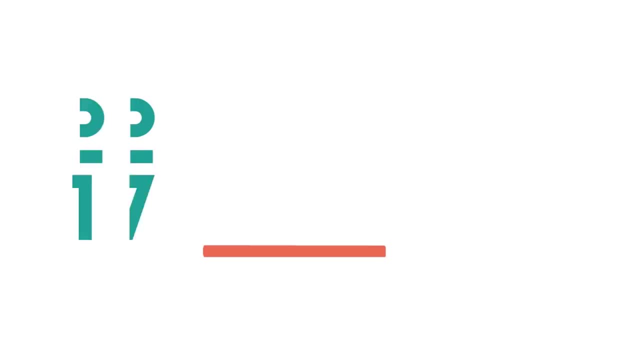 Here we'll show. you Say we have this subtraction problem: 22 minus 17.. Let's follow the process. So first we subtract the ones: What is 2 minus 7?? Well, here's that interesting thing we mentioned to you Say I have 2 carats and I need to give 7 carats away. That's a problem. 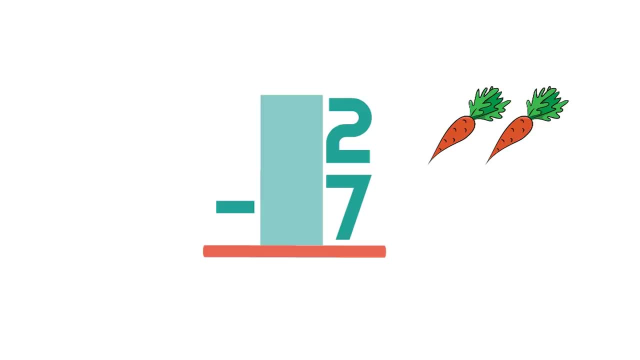 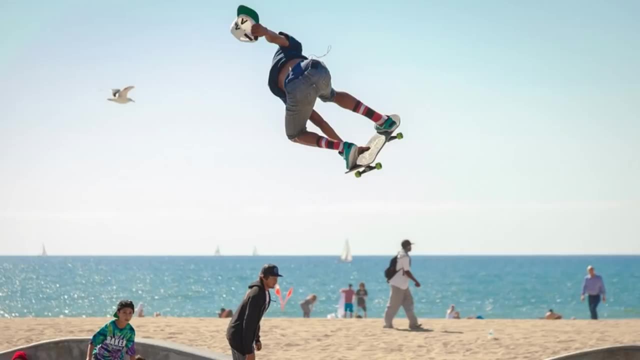 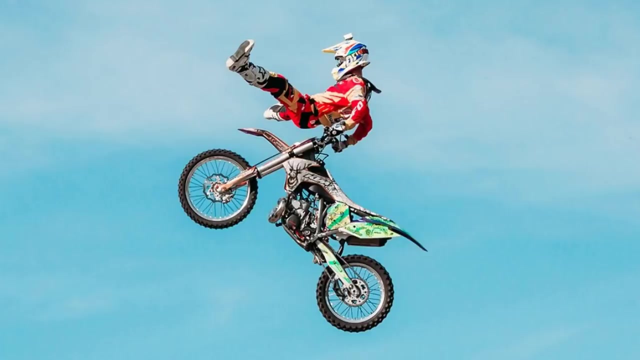 It's hard to give away more than you have. So what do we do? Well, we do a special trick. No, not the same trick, Not this kind of trick. Wow, he is really high up there. No, not this kind of trick either. alright, It's a math trick. okay, It's a math trick. This is a subtraction video, after all. 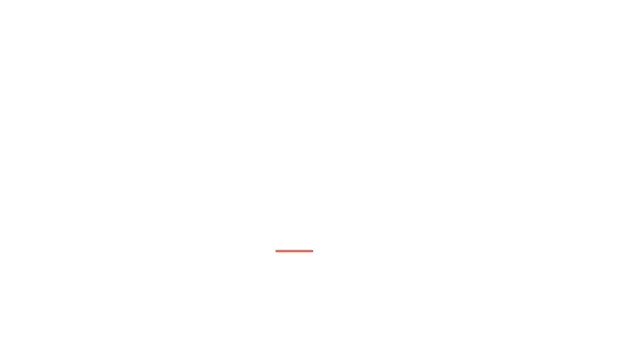 Here we'll show. you Say: we have this subtraction problem: 22 minus 17.. Let's follow the process. So first we subtract the ones: What is 2 minus 7?? Well, here's that interesting thing we mentioned to you Say: I have 2 carrots and I need to. 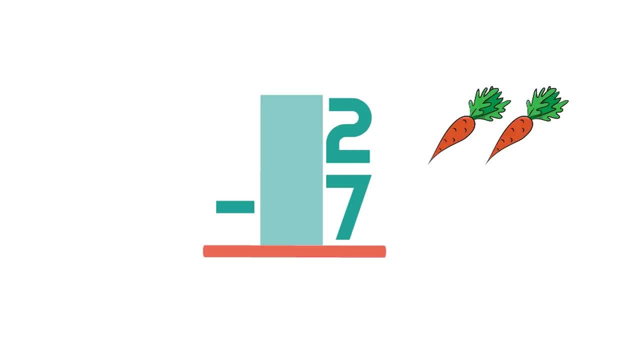 give 7 carrots away. That's a problem. It's hard to give away more than you have. So what do we do? Well, we do a special trick. No, No, not this kind of trick. Wow, he is really high up there. 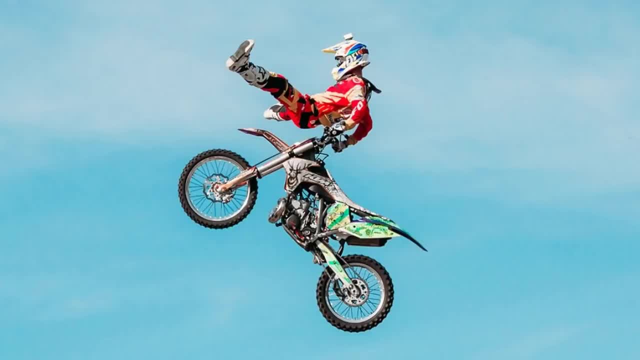 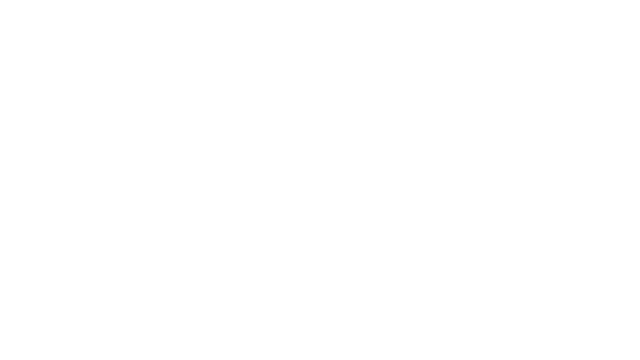 No, not this kind of trick either. Alright, It's a math trick. Okay, It's a math trick. This is a subtraction video. after all, The trick is called regrouping. Can you say that, Regrouping? 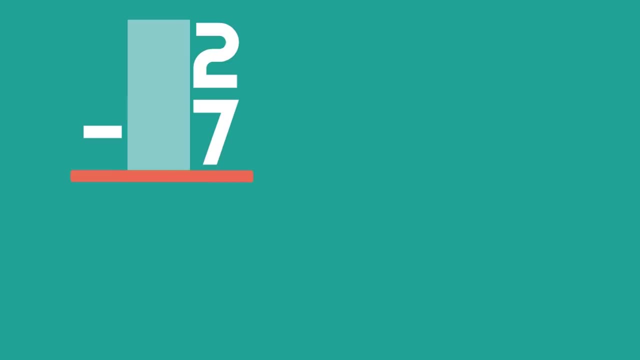 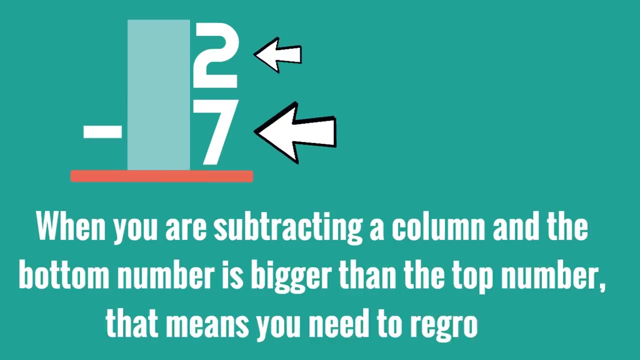 Yeah, Regrouping. When you are subtracting a column and the bottom number is bigger than the total units, it is a subtraction problem. Subtract the left, the grupo, odd the ones bigger than the top number. That means you need to regroup, just like in this example, because it is. 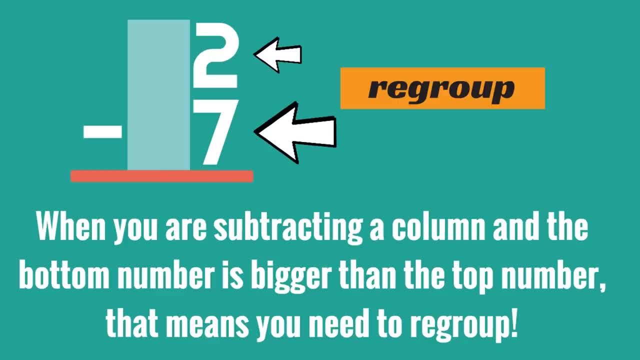 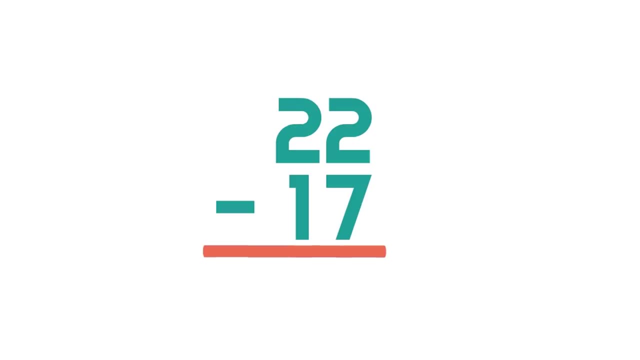 hard to take away more than you have, and 7 is bigger than 2, so we need to regroup. So how does this regrouping trick work? It's really easy. All you do is borrow 1 from the 10s column. What is 2 minus 1?? Yeah, 1.. So this number in the 10s column becomes a 1,. 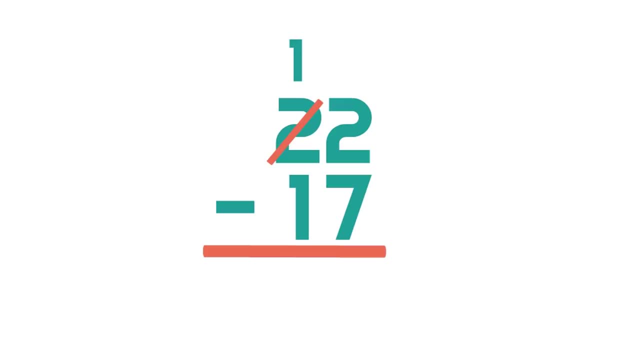 and that 1 that we borrowed from the 10s. it goes to the 1s, it gets placed on this 2 in the 1s column and now the 1s column is 12 minus 7.. Now we just have to follow our subtraction game plan. We subtract the right column, the 1s. 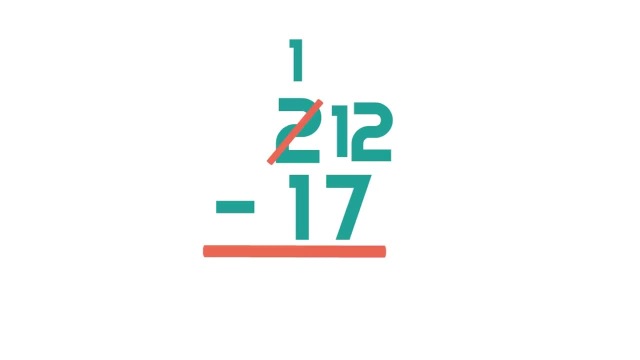 from the 10s column and we subtract the 1s column from the 10s column. First, what is 12 minus 7?? Hmm, Yes, 12 minus 7 equals 5, so we write the number 5 under the. 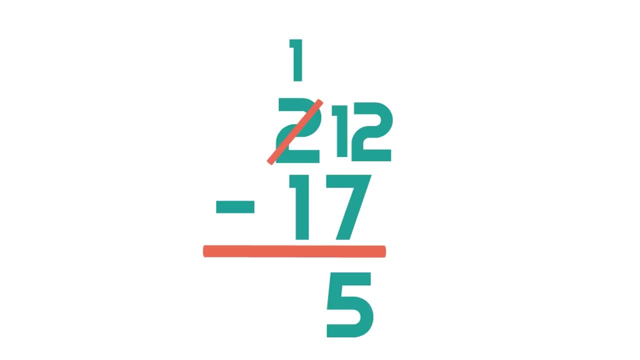 1s column. Then, of course, we have to subtract the 10s, but regrouping made this super easy. What is 1 minus 1?? Yes, 1 minus 1 equals 0, so our answer is simply 5.. 5 is our. 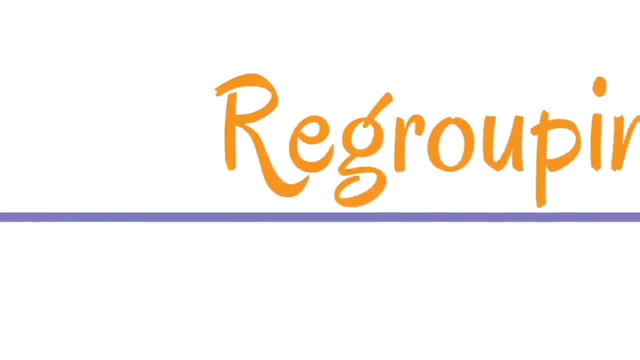 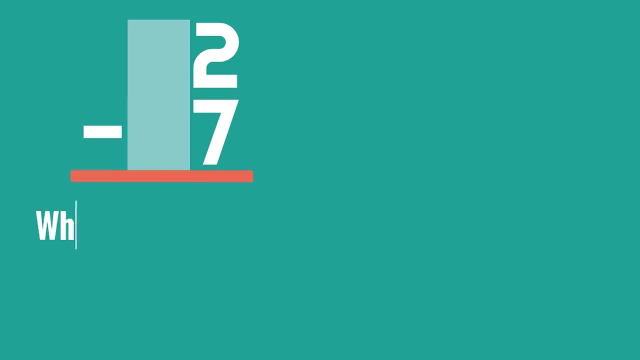 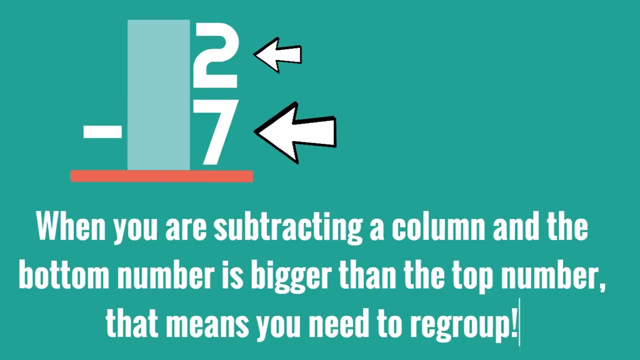 The trick is called regrouping. Can you say that? Regrouping, Yeah, regrouping. When you are subtracting a column and the bottom number is bigger than the top number, that means you need to regroup, Just like in this example, because it is hard to take away more than you have. 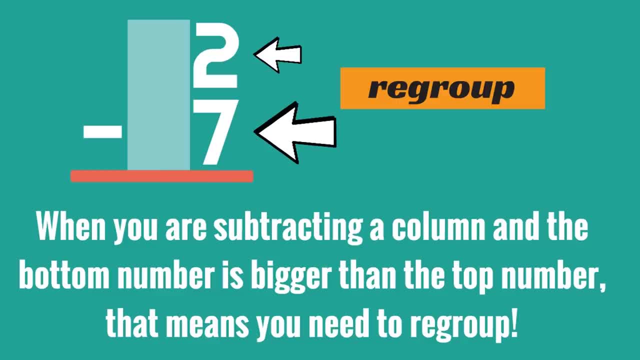 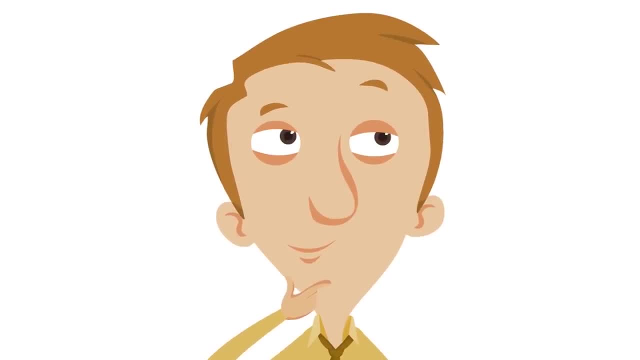 And 7 is bigger than 2.. So we need to regroup. So how does this regrouping trick work? It's really easy. All you do is borrow 1 from the tens column. What is 2 minus 1?? Yeah, 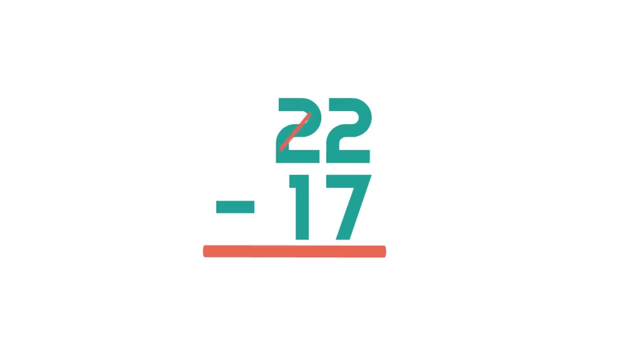 1.. So this number in the tens column becomes a 1. And that 1 that we borrowed from the tens, it goes to the 1s. It gets placed on this 2 in the 1s column And now the 1s column is 12 minus 7.. 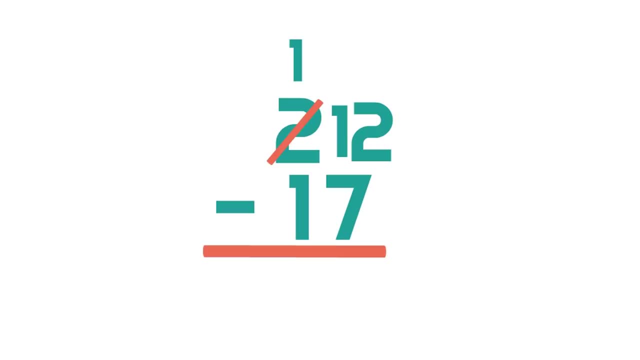 Now we just have to follow our subtraction game plan. We subtract the right column, the 1s, first. What is 12 minus 7?? Hmm, Yes, 12 minus 7 equals 5.. So we write the number 5 under the 1s column. Then, of course, we have to subtract the tens. 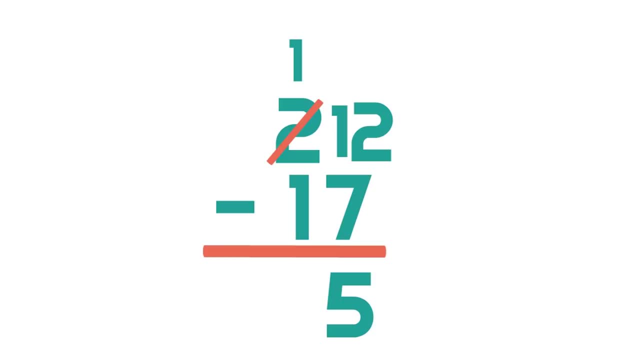 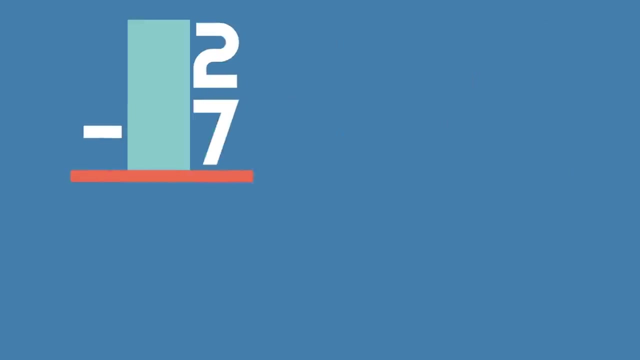 But regrouping made this super easy. What is 1 minus 1?? Yes, 1 minus 1 equals 0. So our answer is simply 5.. 5 is our difference. Remember when you are subtracting a column and the bottom number is bigger than the top. 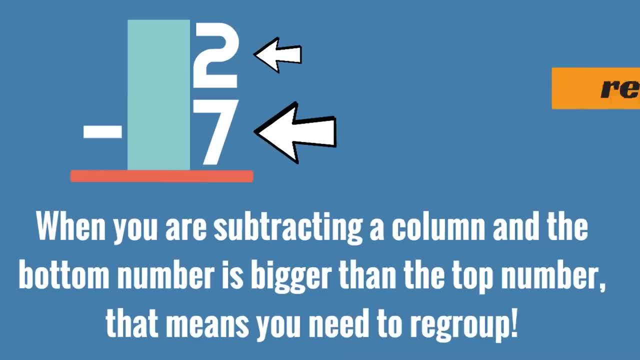 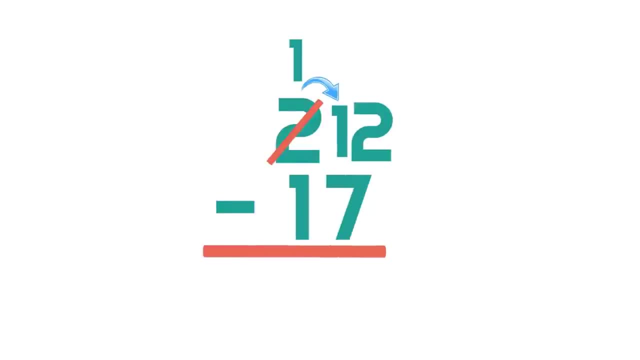 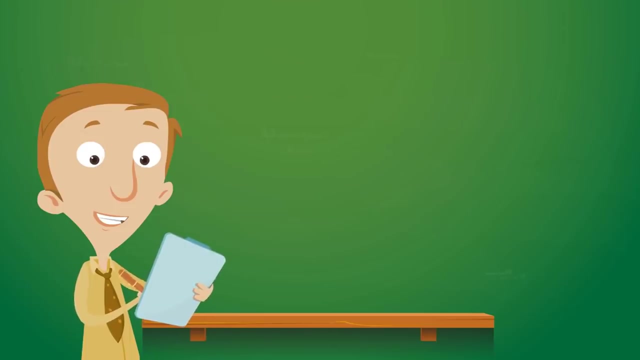 number, that means you need to regroup and with subtraction regrouping means borrowing In double digit. subtraction. regrouping is when you borrow one from the tens column. Let's try one more double digit subtraction problem and see if we need to use the special. 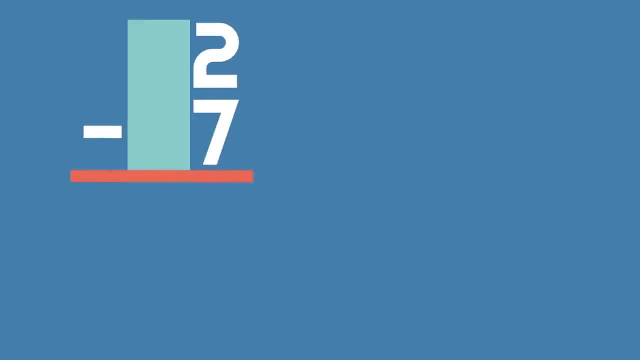 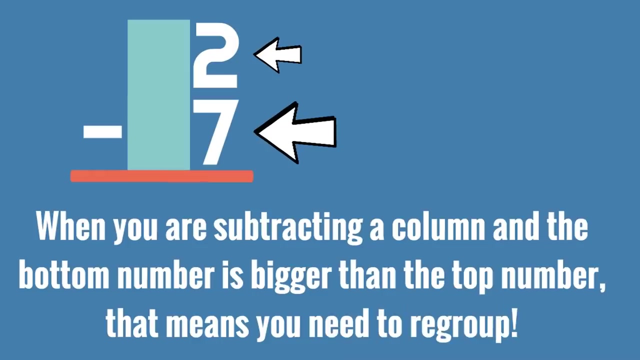 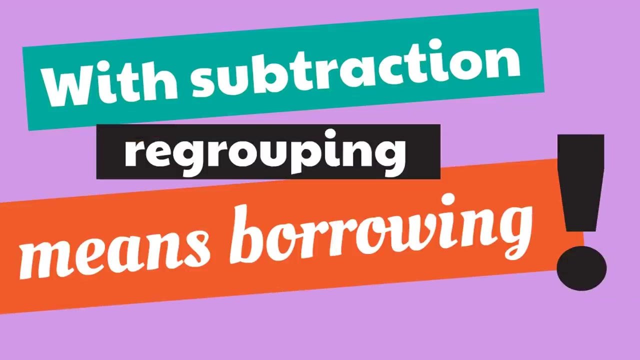 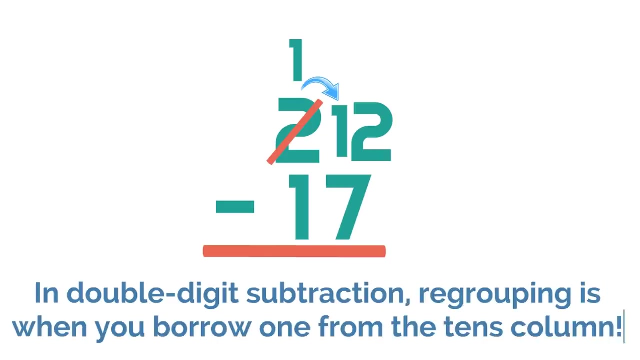 difference. Remember, when you are subtracting a column and the bottom number is bigger than the top number, that means you need to regroup and with subtraction, regrouping means borrowing In double-digit subtraction. regrouping is when you borrow 1 from the 10s column. 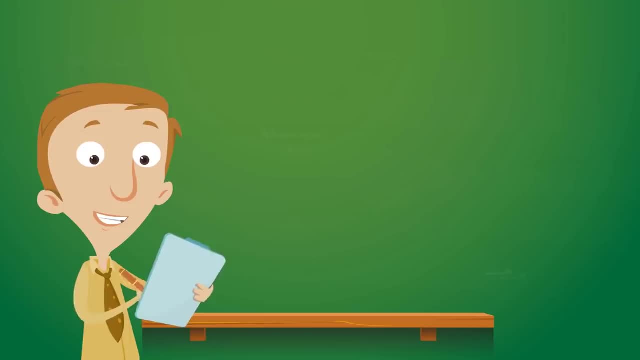 Let's try one more double-digit subtraction problem. Let's try one more double-digit subtraction problem. Let's try one more double-digit subtraction problem and see if we need to use the special regrouping trick: 43 minus 25.. This is going to be awesome. Remember the first thing we 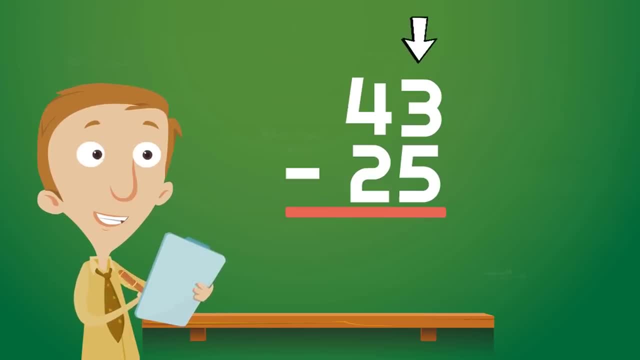 do is subtract the right column, the 1s, but uh-oh 5, the bottom digit is bigger than 3, the top digit Time to regroup, So we borrow 1 from the 10s column. What is 4 minus 1?? 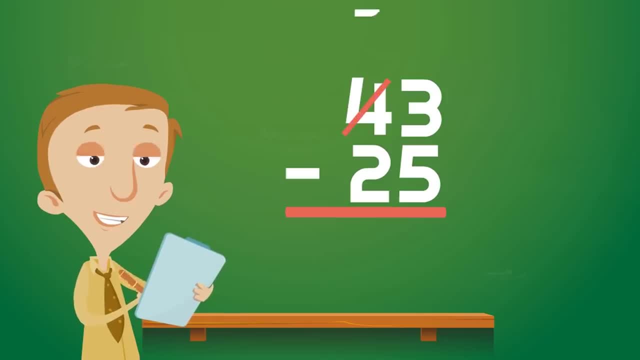 Yes, 3.. Then we put that 1 in front of the 3 in the 1s column, making it the number 13.. Then we just follow the process, subtracting the 1s column first, What is 13 minus 5?? 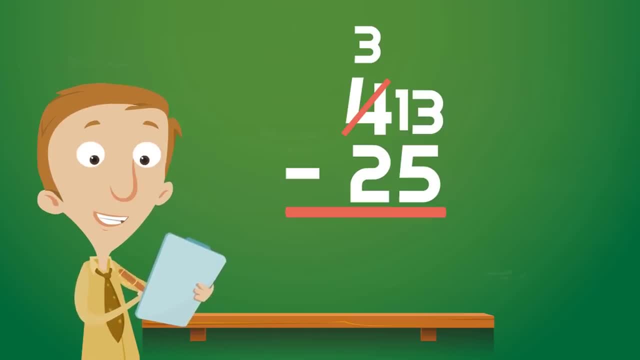 What is 13 minus 5?? Yep, it is 8.. So we will write 8 under the 1s column. Now it's time to subtract the 10s. What is 3 minus 2?? What is 3 minus 2?? You got it: 3 minus 2 equals 1.. So we put the number 1 under the 10s column. 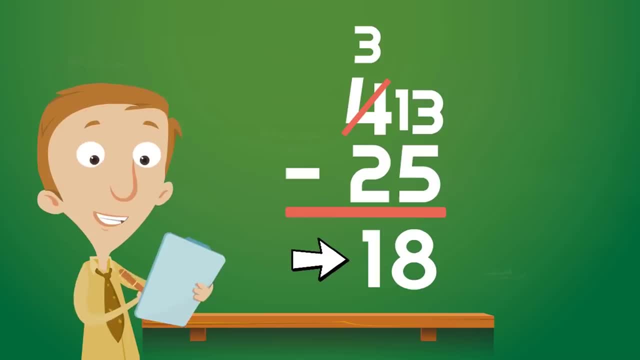 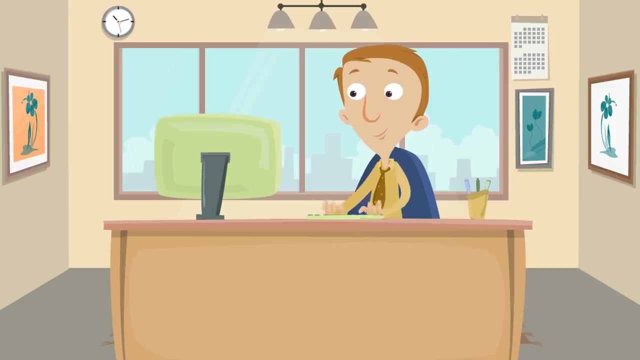 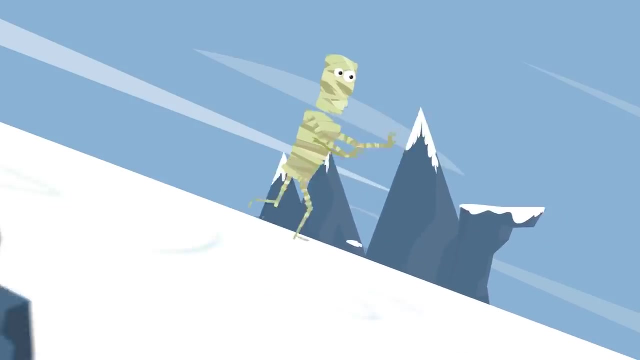 and we have our answer: 43 minus 25 equals 18.. 18 is the difference. We've learned a lot, but we need to make sure we are able to remember everything. Here's an idea. There's this guy, Mummy, who doesn't know how to do double-digit subtraction- okay. 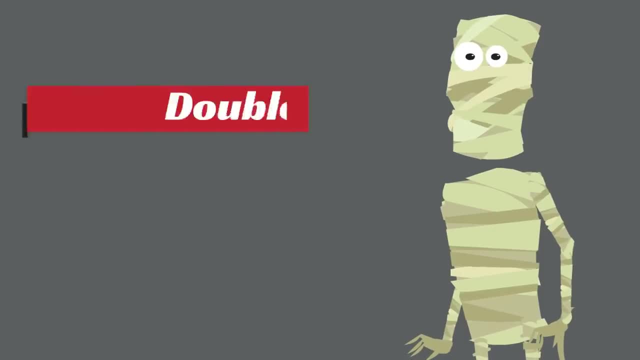 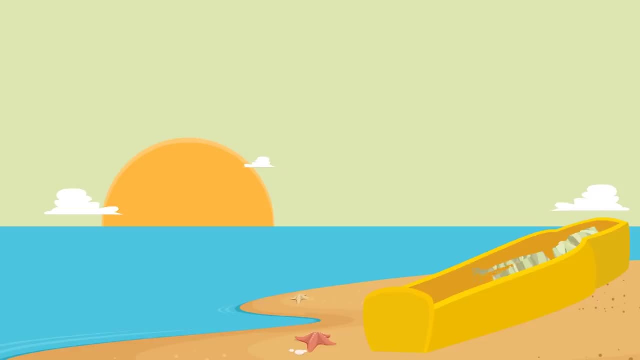 So we are going to do a double-digit subtraction review by teaching Mummy: It's simple and it's fun, Mummy, You'll love it. So, Mummy, subtraction is when you take numbers way. sometimes subtraction problems can have little numbers, or other times subtraction problems can. 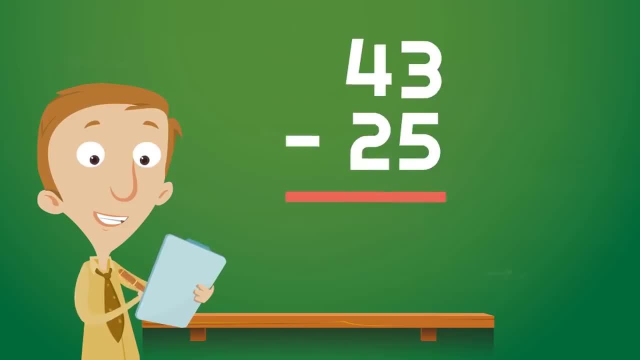 regrouping trick: 43 minus 25.. This is going to be awesome, Remember. the first thing we do is subtract the right column, the ones. but uh oh, five. the bottom digit is bigger than three. the top digit. 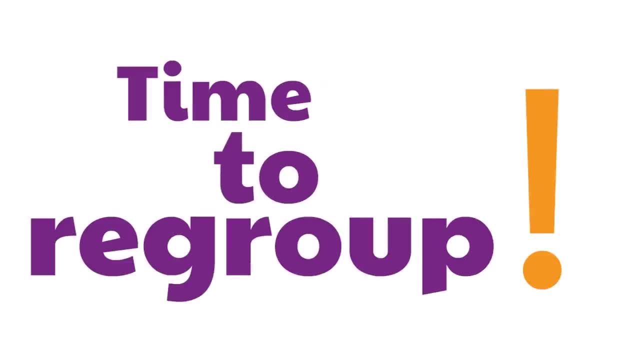 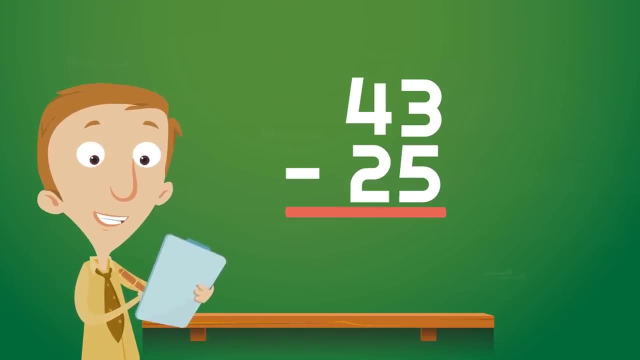 Time to regroup. So we borrow one from the tens column. What is four minus one? Yes, three. Then we put that one in front of the three in the ones column, making it the number 13.. Then we just follow the process subtracting the ones column first. 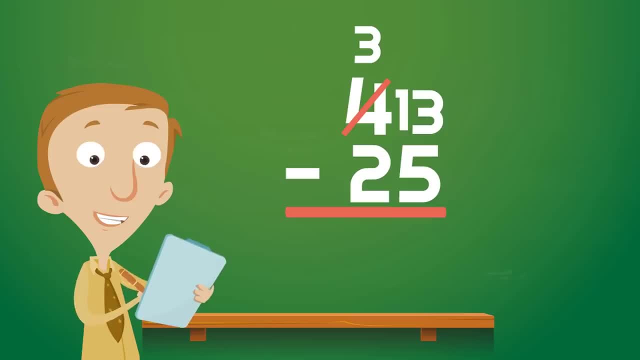 What is 13 minus five? What is 13 minus five? Yep, It is eight. So we will write eight under the ones column. Now it's time to subtract the tens. What is three minus two? What is three minus two? 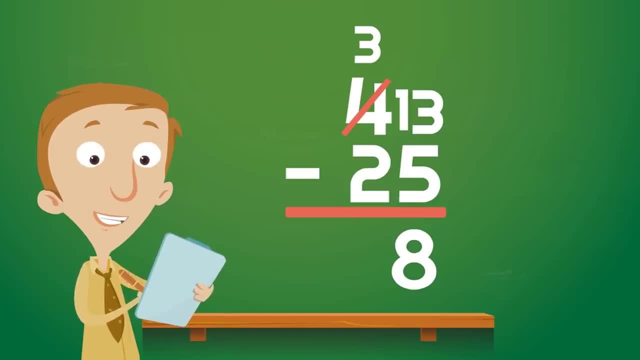 You got it. Three minus two equals one. So we put the number one under the tens column and we have our answer: 43 minus 25 equals 18.. 18 is the number. That's right, That's the number. What is the difference? 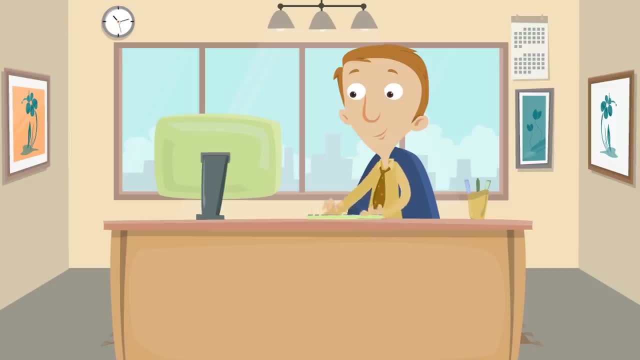 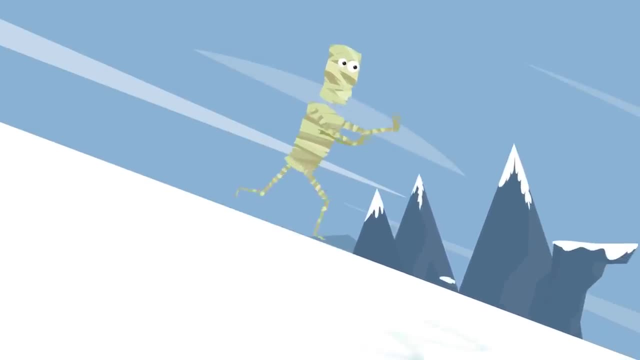 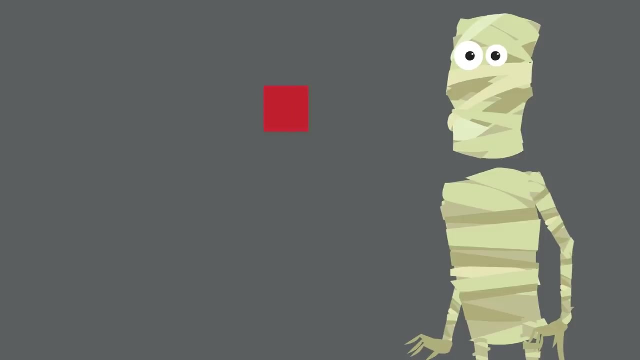 We've learned a lot, but we need to make sure we are able to remember everything. Here's an idea. There's this guy, mummy, who doesn't know how to do double digit subtraction. Okay, so we are going to do a double digit subtraction review by teaching mummy. 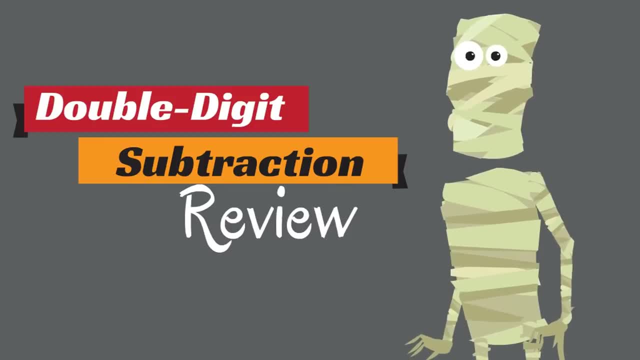 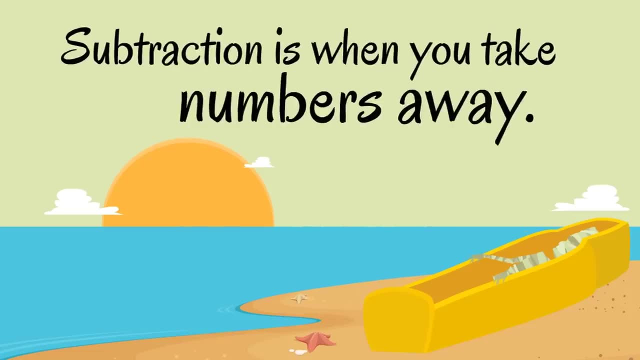 It's simple and it's fun, Mummy, You'll love it. OK. So, Mummy, subtraction is when you take numbers away. Sometimes subtraction problems can have little numbers, or other times subtraction problems can have bigger numbers, double-digit numbers. 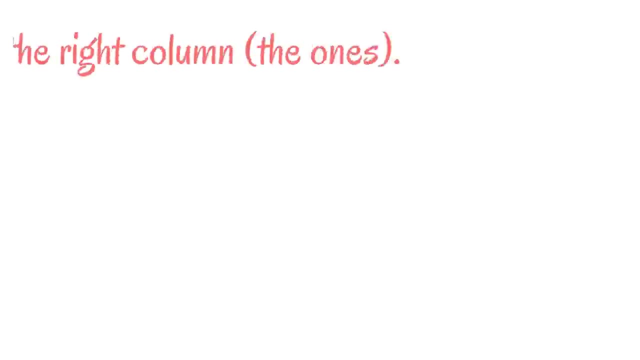 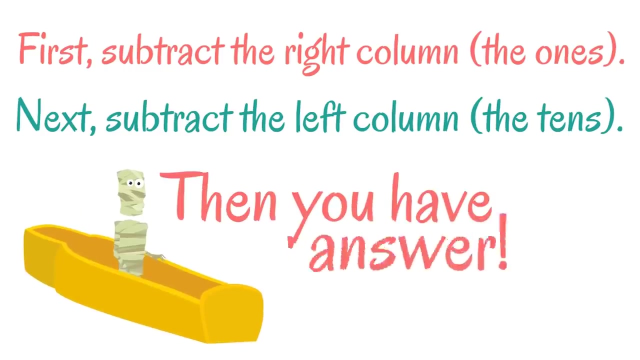 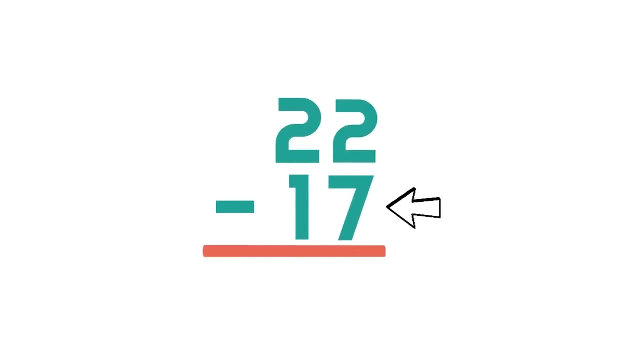 Here's how it works, Mummy: First subtract the right column, the ones. Next you subtract the left column, the tens. Then you have your answer, which is called the difference. Sometimes the bottom digit is bigger than the top digit in the ones column.